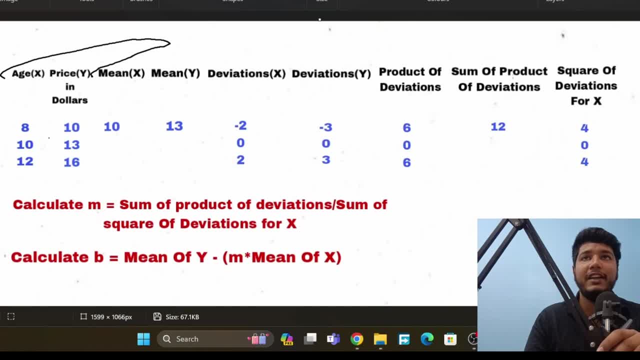 is equal to 10. so we will same for the mean of y. we will add the value of y here, price, which is, and then we will divide it by 3, so the value is 13. so now we have to calculate deviation. so deviation in we have to do is that first we will calculate deviation of 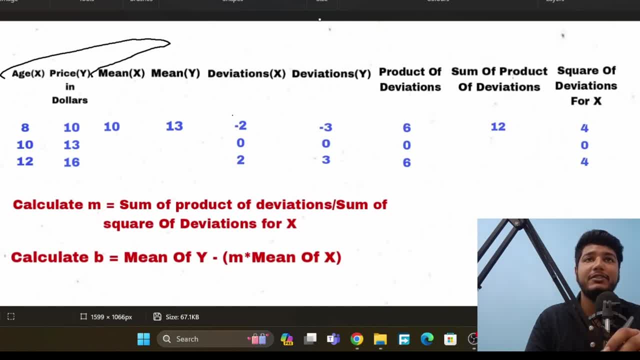 x, so we will minus 8 minus 10.. Which is equal to minus 2, 10 minus 13 is equal to 2 and 0 means and 12 minus 16 is equal to 2 and same. we will do with deviation y, which is 10 minus 13 is equal to minus 3. 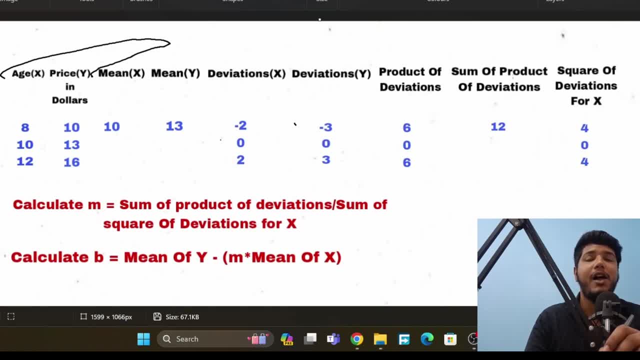 and so all 13 minus 13 is equal to 0, 60 minus 13 is equal to 3, and now we will do product of deviations. so we will multiply this x and deviation x and deviation y, which is, we will multiply it here. 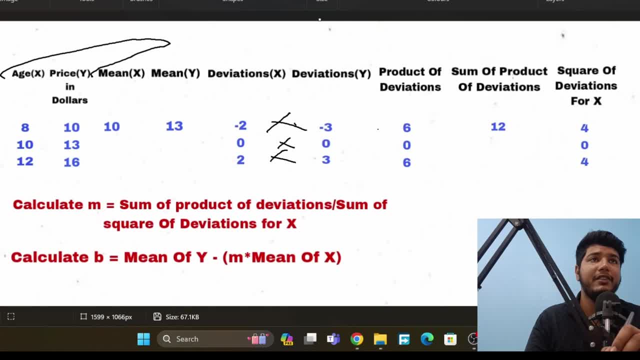 Like this: all 3, and the value we get here is minus minus plus 6, 0, 6, and we will do next sum of product of deviation. so we will plus it all, so the value we get is 12. next we will do square of deviation for x. so here what we will do is we will square x, so deviation. 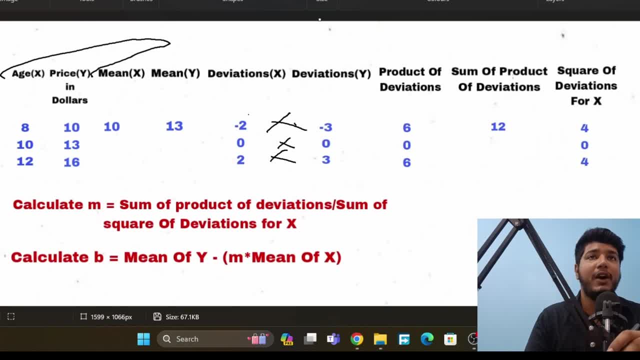 x. so minus 2, minus 2 in square is equal to minus 2, square is equal to 4 because it is in plus, Because zero square is equal to zero here and 2 square is equal to 4. so here we have done this much stuff. 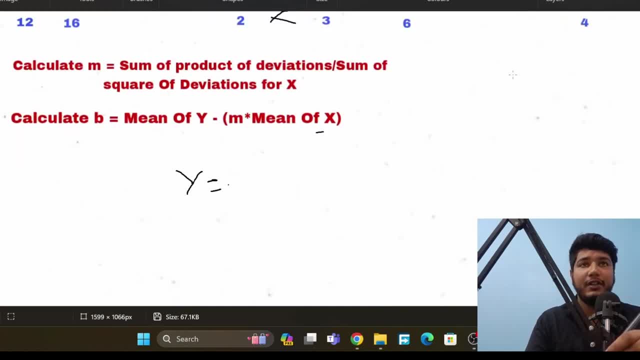 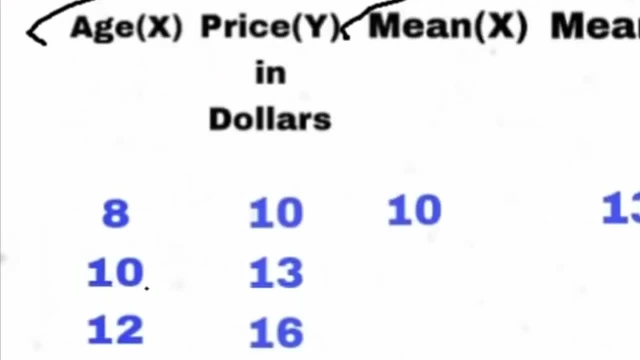 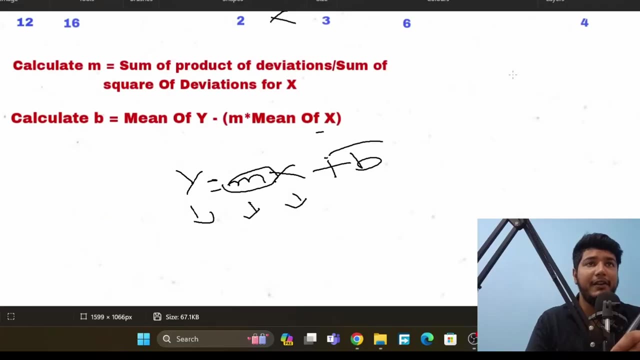 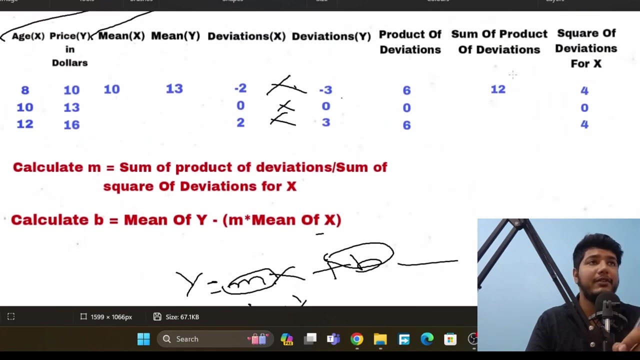 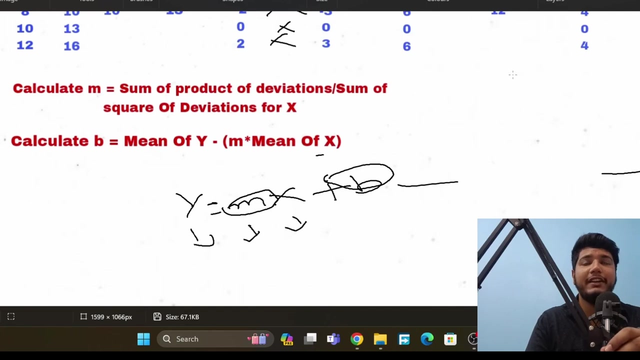 So here is our equation: y is equal to mx plus b. so here we have our y already, and we have already and we have to calculate m and b. so here you can see that y and x is there. okay, y is here, our x is here. okay, now we will calculate m and b. so, in order to calculate m, 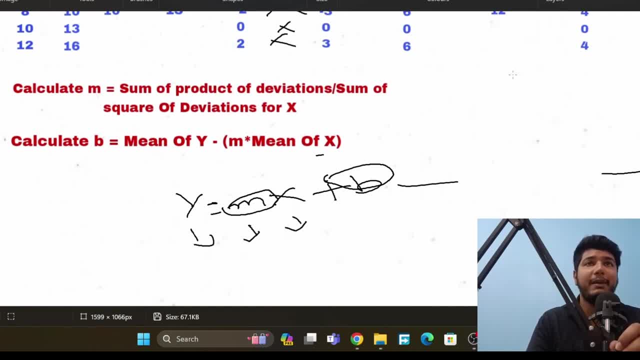 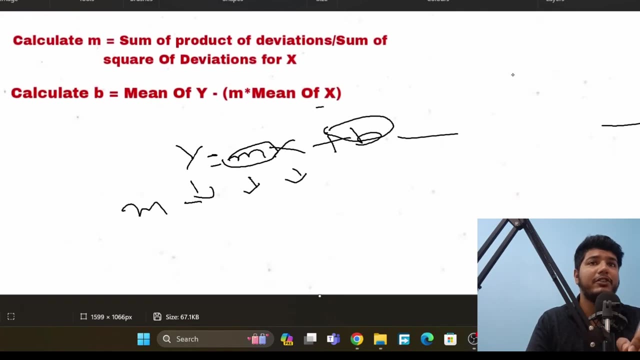 this is the formula: sum of product of deviations divided by sum of square of deviation for x. so so here we will do here m. so what is the sum of product of deviation? let's look: sum of product of deviation is equal to 12, 12 divided by. 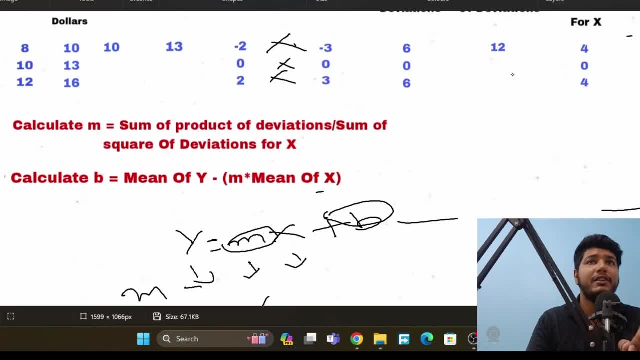 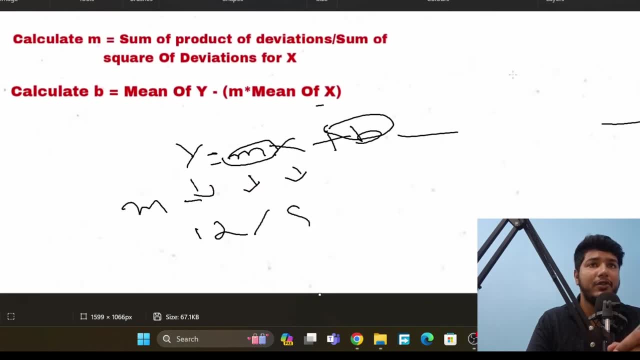 8, which is sum of product of square of deviation. so we will plus it all here. so which is the value, our 8? so we will divide it. so when we divide it, what value we get? we get 1.5. okay, now we have done here. now we will calculate b. b is equal to mean of y. 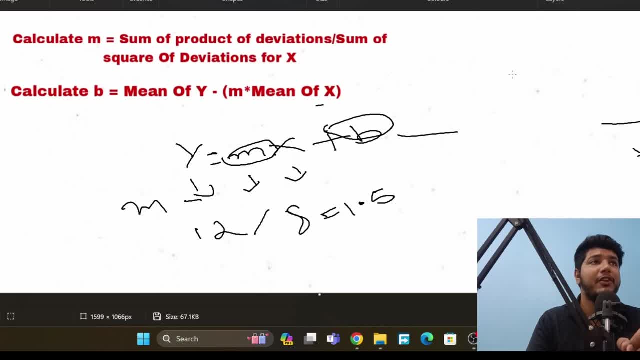 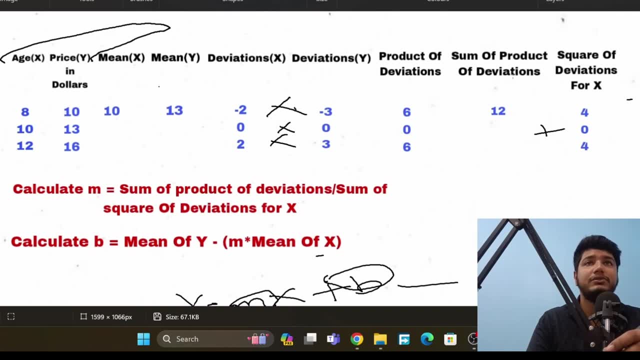 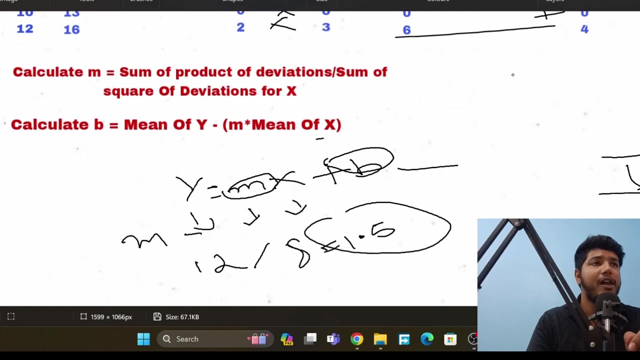 so now, what's p or y? so it is p to the power of f and m minus m into mean of x. so what is mean of y? let's show you here. so mean of y. so this is mean of y, this is 13, and m and m is about this. we have 1.5, which have? we have calculated. 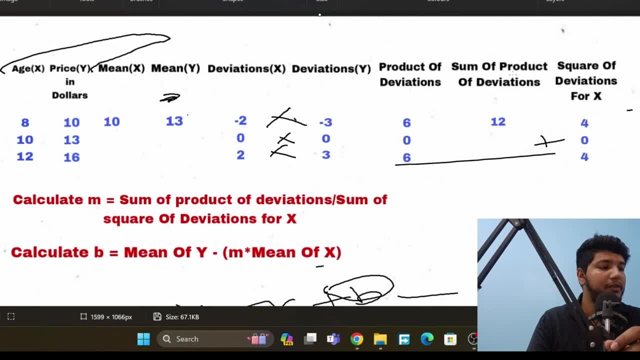 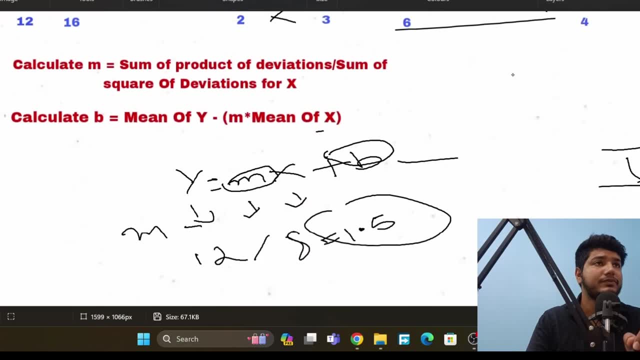 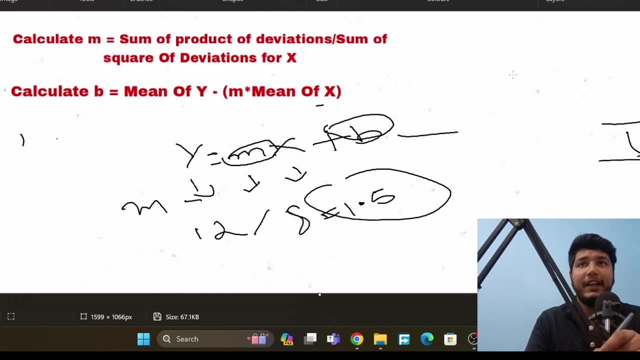 here. you can see here, 1.5 is our, and to multiply it with mean of x, which is 10, so let's do it. sorry for writing like this, but i am not used to use graphic tablets, so here is 13 minus 1.5 in bracket into 10, 13. 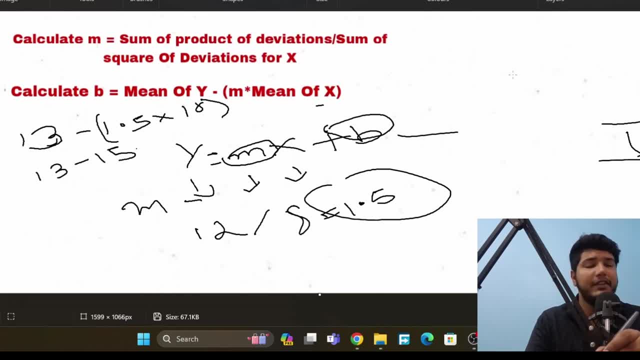 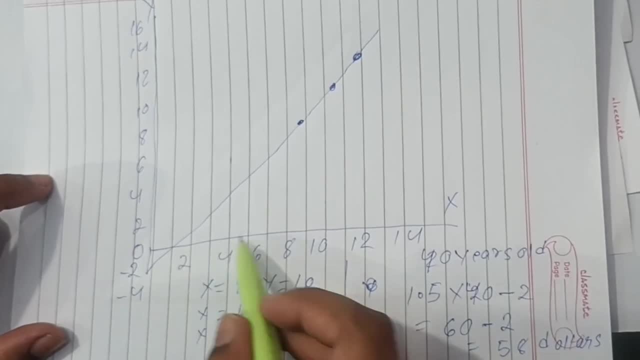 minus 5, 15 is equal to minus 2. so here we have done, we have find a, b and now we will visualize it. so let's visualize it. so now we have get the b, so this means that we will visualize it now. so i have visualized it. you can see this here. so x is equal to 0 when 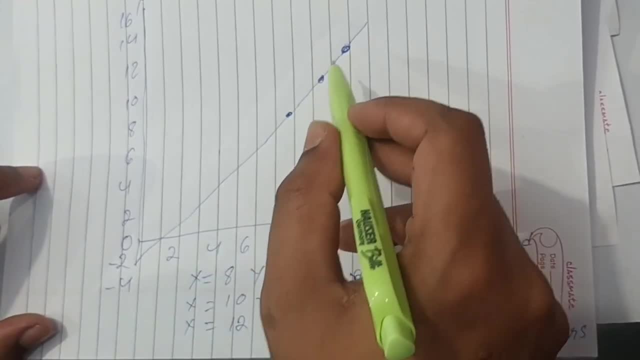 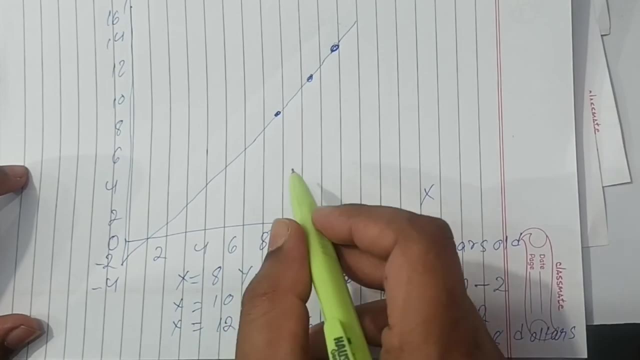 x is equal to 0, y is equal to minus 2, so i have visualized it by positive regression. and here you have the, the price we have gotten and age we have gotten. i have showed it here. so x is equal to 8 and y is equal to 10. so